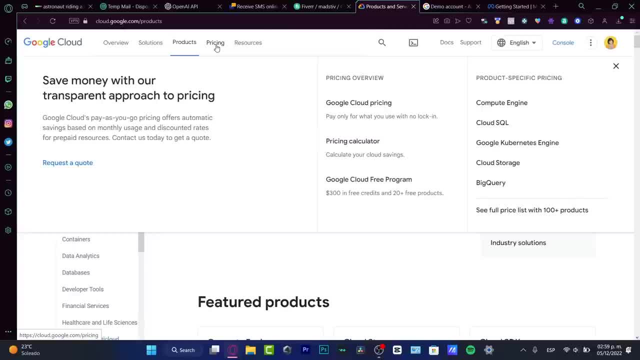 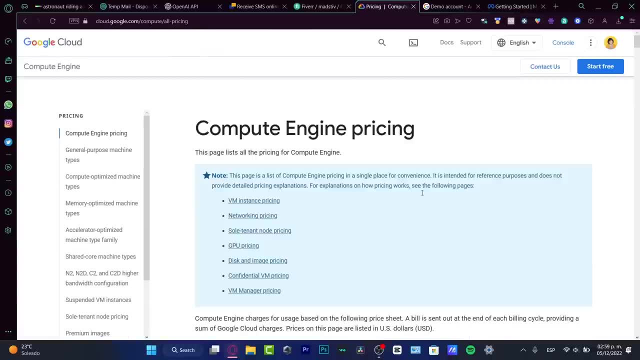 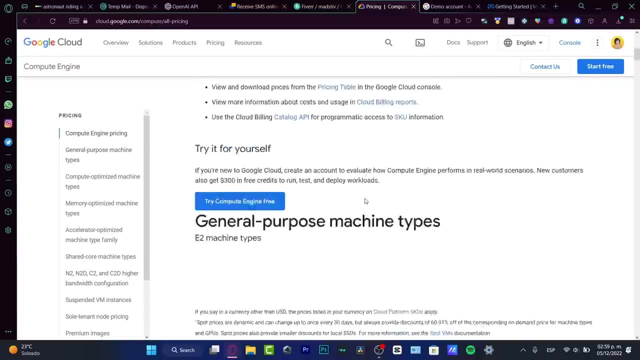 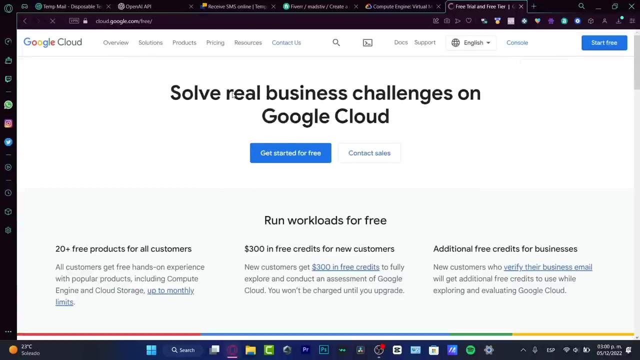 order to see what we can do like totally for free, I went into the Google pricing And actually I was trying to look for a tire And I realized that there's actually a tire that is actually for free. So here, what I'm going to be choosing here is this option of GCP, And here we have this overall business challenges. I'm going to be screwing a little bit down, As you can see. this one is the. 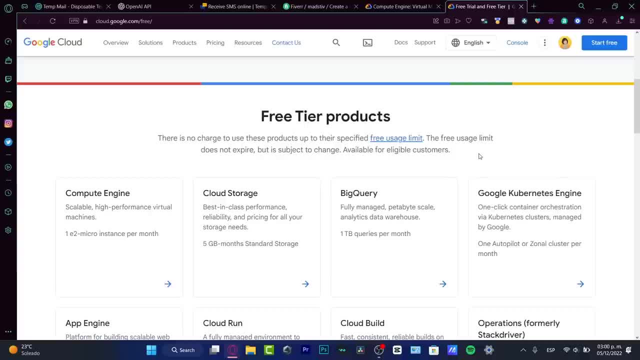 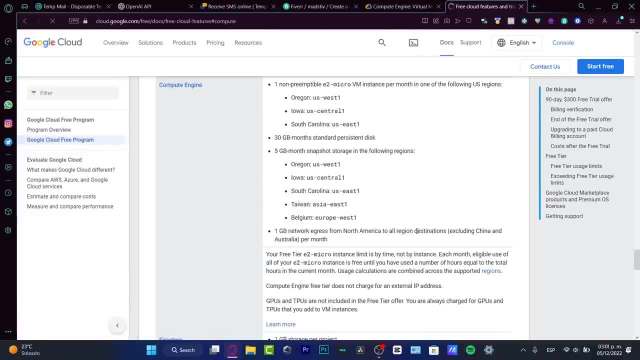 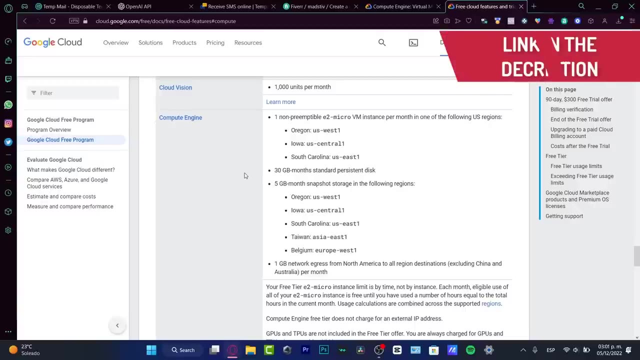 GCP, And here we have this overall business challenges. I'm going to be screwing a little bit down, As you can see. this one is the option that we was looking for, the free trial product. So if I head into the compute engine of the cloud storage, you can with this during this later. here we have the requirements in order to get this for free. So this is what we are looking for: free thoughts, free tire tier. So here I have the known, imprimptible ETU micro BM, instant and instant per month in one. 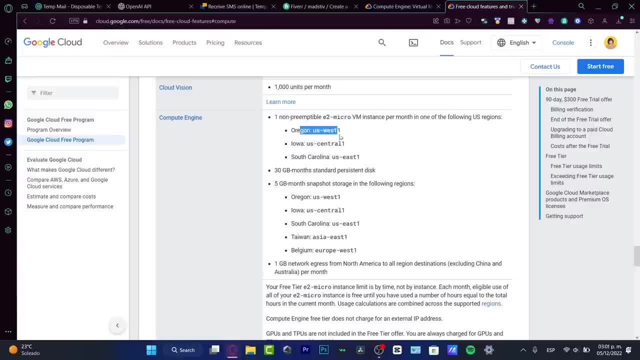 of the following US regions. so I'm going to be choosing the US West one or the Iowa or the South Carolina. so I need to provide all of this information in order to get a free tire. free tire, so you need to hit into start free. so here you want. 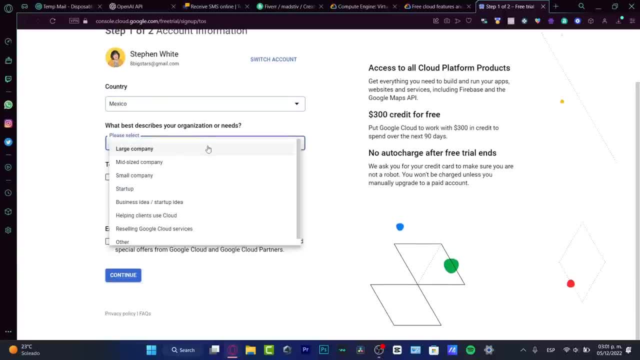 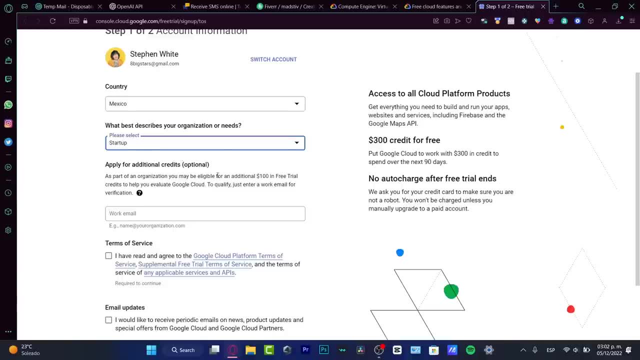 to choose your country. what best describes your organization or needs? so let's say that this is just a startup. apply for additional credits as part of an organization. you may be eligible for additional a hundred free trial credit to help you. every lady, Google account and cloud to qualify. we don't want to. 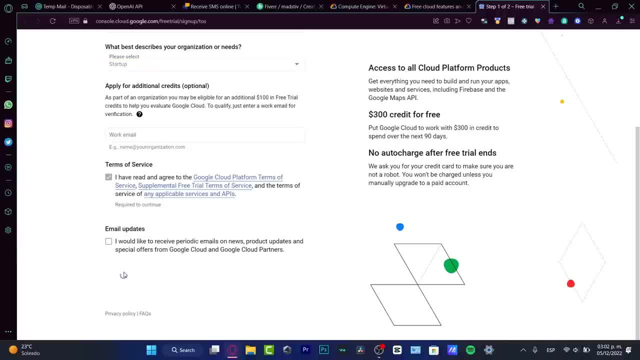 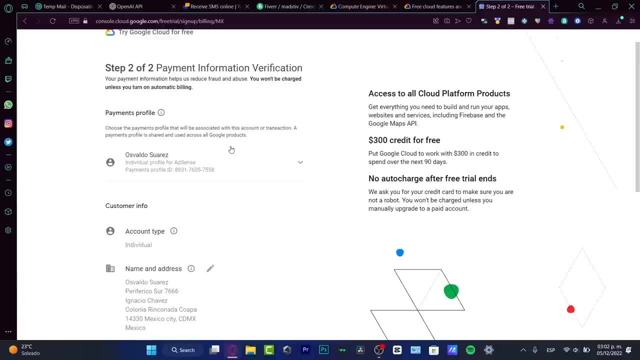 focus in here once you agree to the terms and service and hit into continue. I don't want to mess around in here because we are just getting started right. so we do have a free trial option. as you can see, I have a premium profile already added as an AdSense. if you don't have an account of that, it's gonna be. 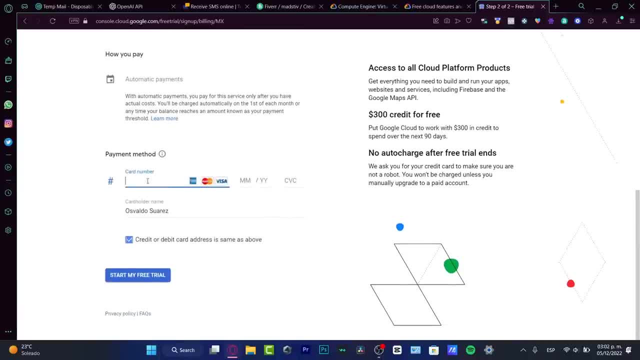 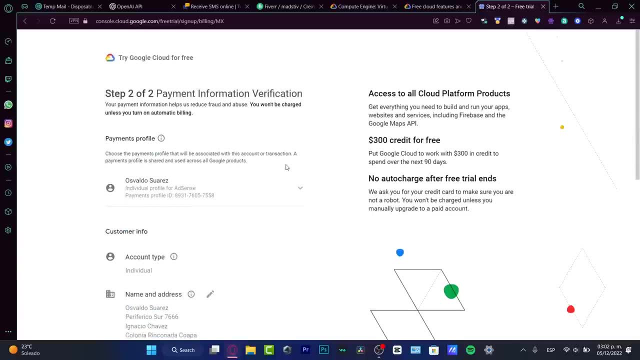 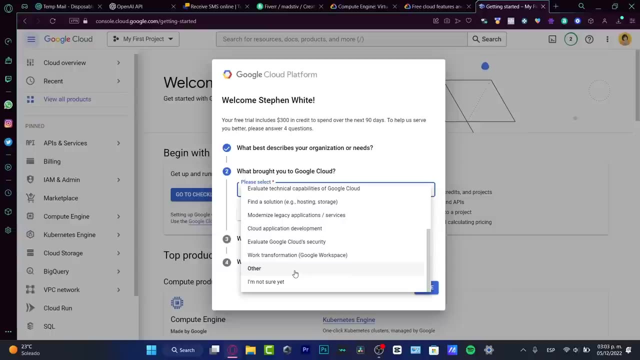 helping you to create it like right away. so we do have the payment method of the, of this option, of the cry of the try Google crowd for free. so what brought us to the Google cloud? so we want to host a website, right. so I'm going to choose into- I'm not sure yet. 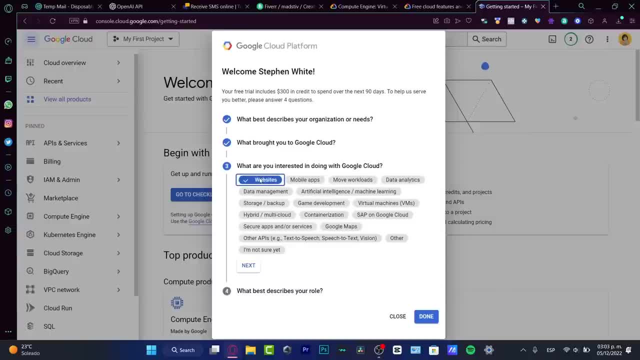 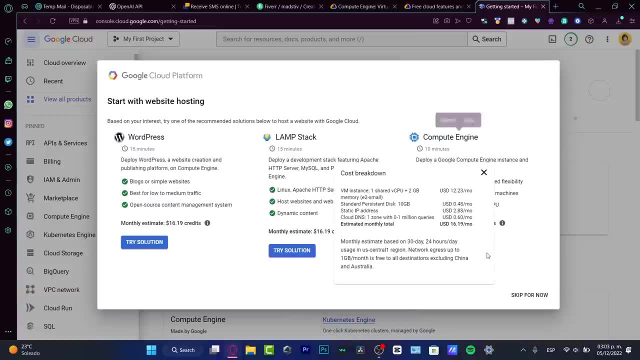 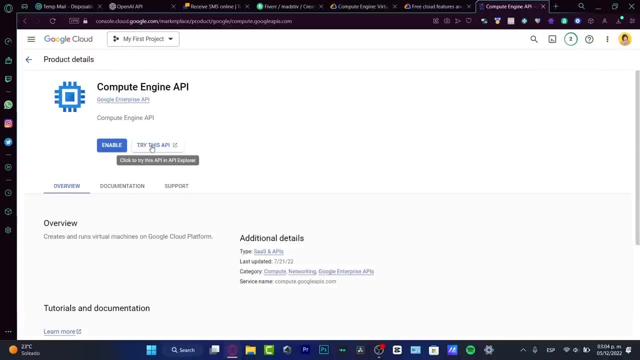 hit into next. what are you interested in doing? kids websites- go into done. and this is the computer engine. so I'm gonna hit into try solution. I need to go to go to computer engine, which is actually like really, really simple. you don't have to be focused in a line here. so once we are here, we want to enable the compute. 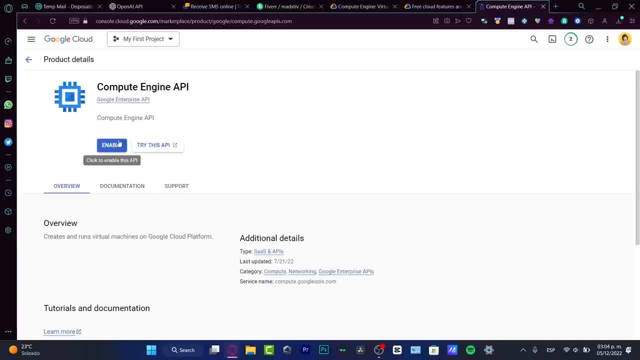 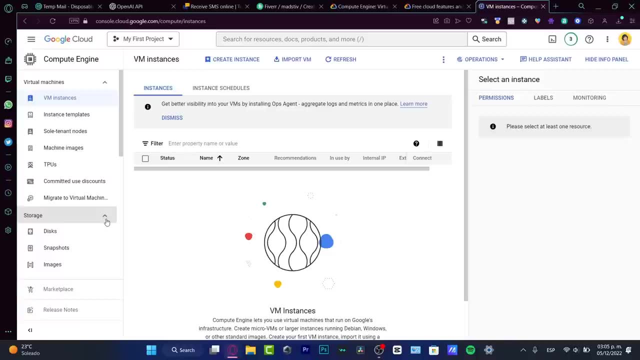 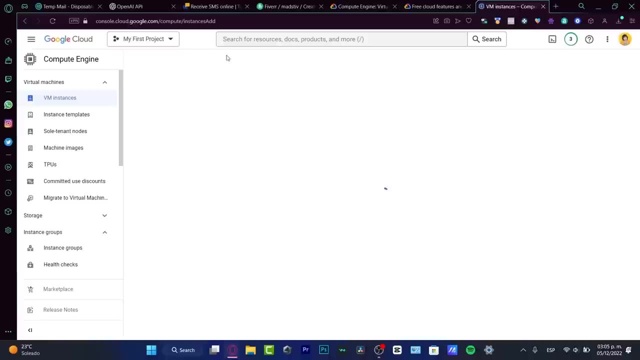 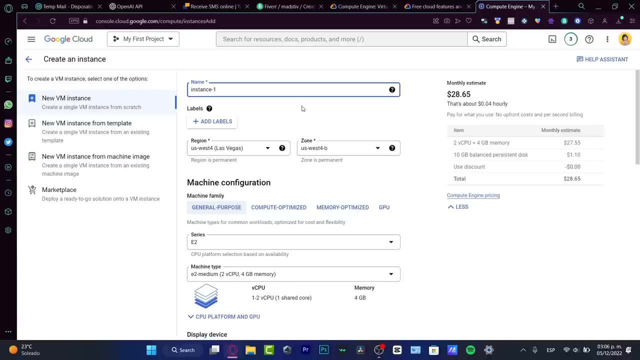 engine API. I'm gonna hit into enable. alright. so here we have the BM instances, we have the template, we have the machines. what did you want to look for and see? my computer engine is to create my first instance. I want to just wait a few seconds into the instance is going to be creating, helping us to create our BM. 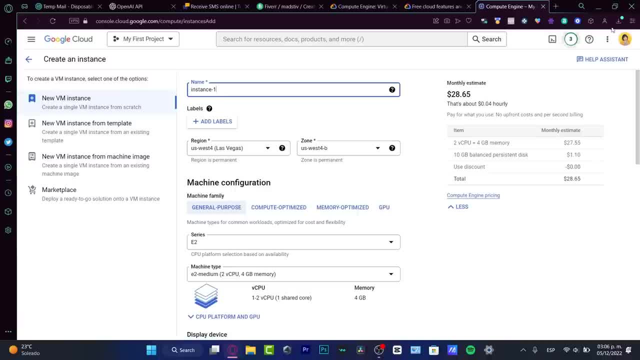 instance, truly from scratch. now, as you can see, I do have a monthly estimate of $28, that's about like 0.04 dollars per hour. so you don't have to be worrying about that, because all of this stuff has been added automatically. so that's the. 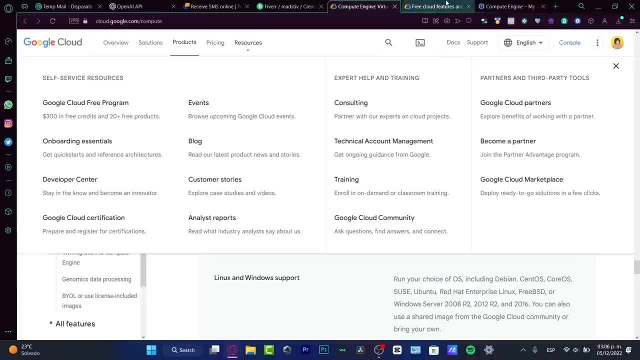 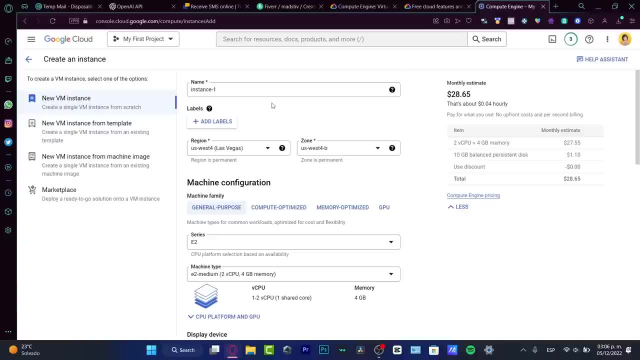 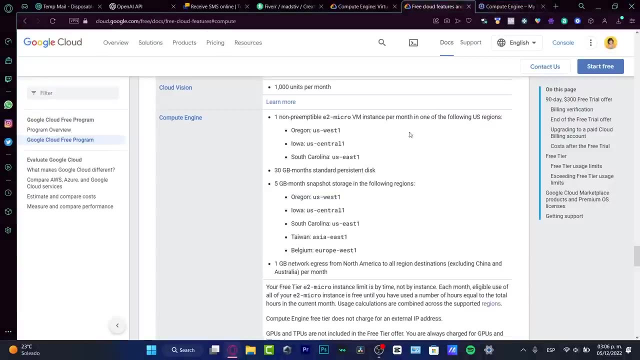 reason. why do you want to have? I actually have this option of the compute engine for free. this is a free tire. so here I do want to look for the regions that are available. so, for example, here I want to look for the US region. I want to look. 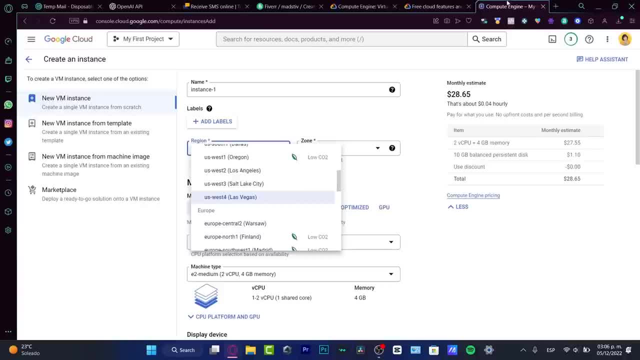 here for the Oregon US West number one. so here I have the Oregon US West number one. you don't want to be focused into the zone and, as you can see, a price: Louis, automatically $25. so that's what we will be looking for. we don't want to pay a. 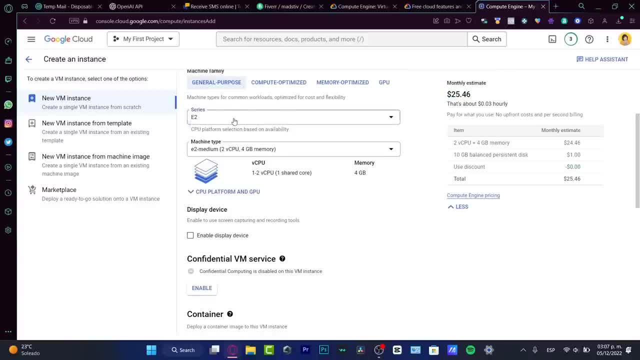 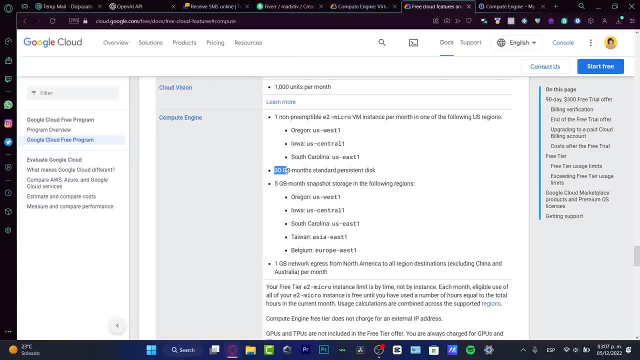 fee for anything right and after that. we do have the series e, number two. let's see if this machine family we need to change the. so we do have a 30 gigabytes moment standard persistent disc. so what you want to do is do once again here. 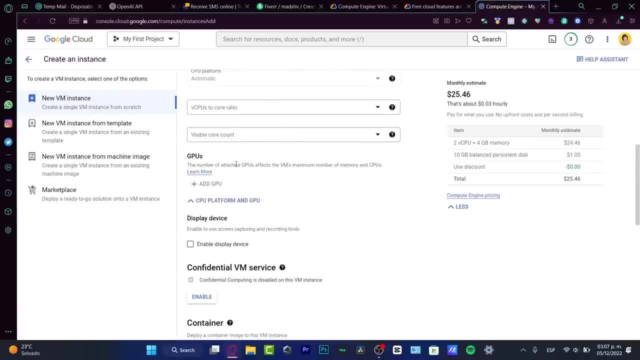 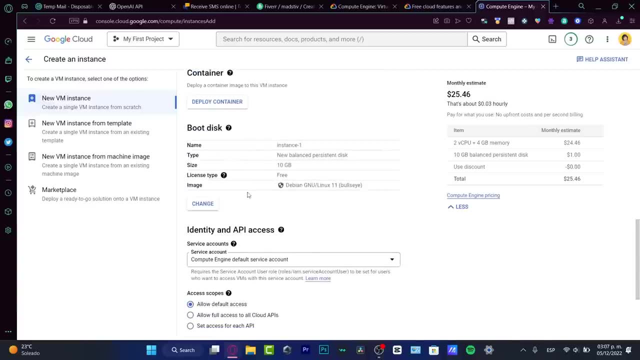 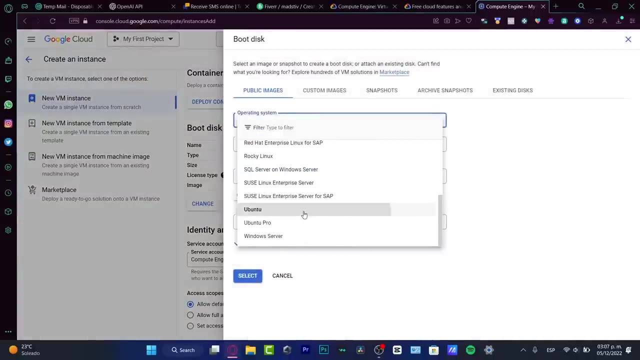 look for that option. I'm going to use a skip, this GPU. I want to skip this for a second. here we have the display device, the confidential BM servers container boot disk, and here want to change it, and here I have the version. I want to scroll my way and look for Ubuntu and here into the 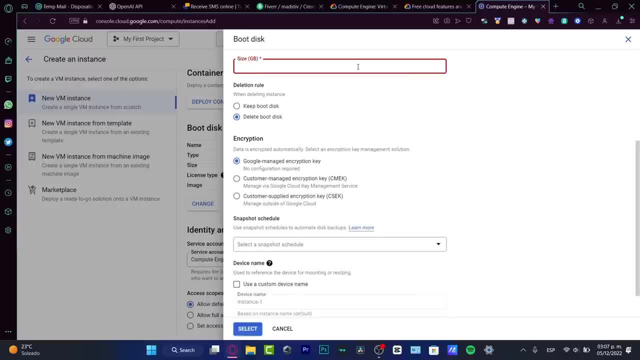 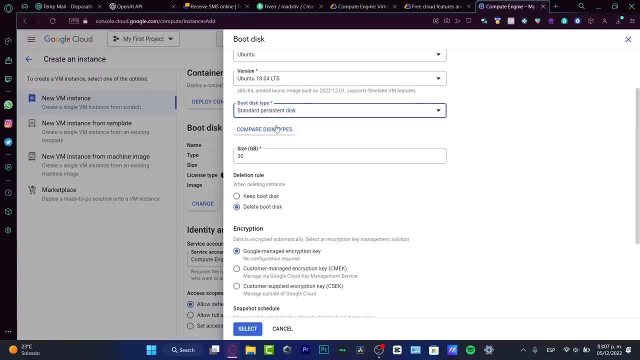 size. I'm pretty sure it was 30 actually, so I'm going to use a little and go into 30.. so there we go, and here I have the balance persistent disk. I want to lose the. I want to look the standard one and go into select. so here, once again, I need. 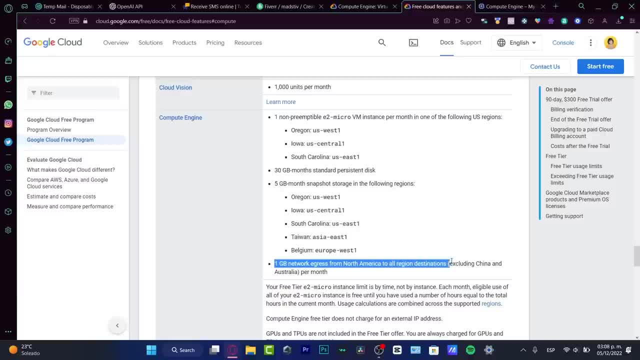 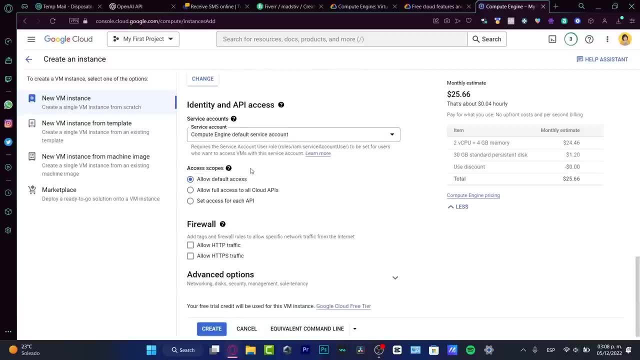 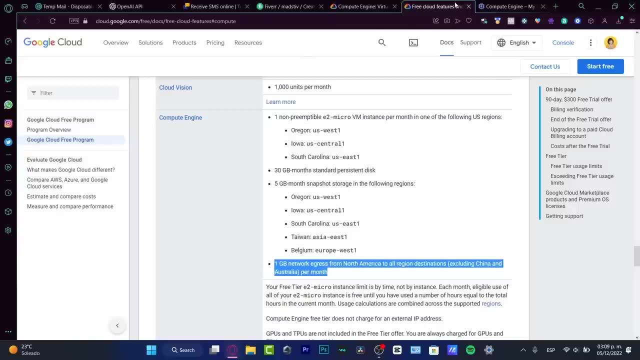 to choose the one gigabyte Network egress from North America, excluding China and Australia, per month. so once again, I just need to go into the firewall advanced options. i'm going to pop this for a second. remember to use the free trial option. so, for example, I do have here at the E2. 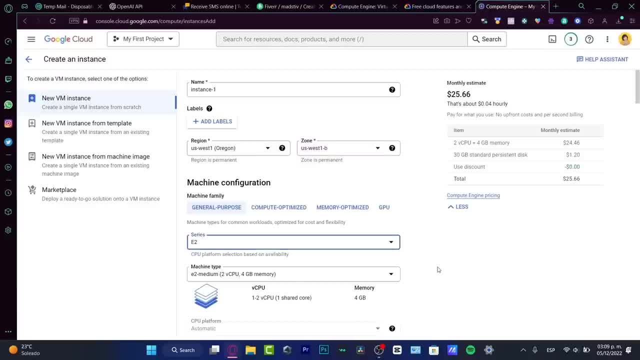 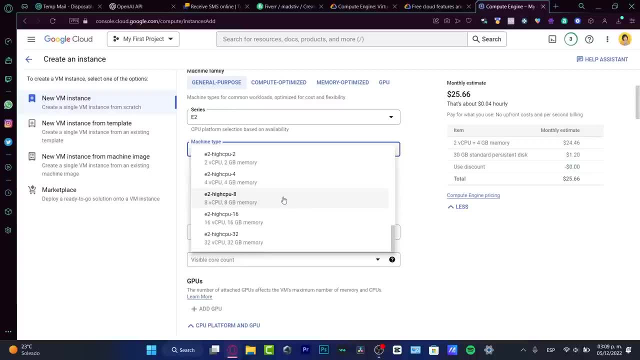 micro instant. so I'm going to go here into the computer engine and need to scroll all my way up until the machine configuration and here I'm going to be choosing the E2 micro limit. so E2 here it is, E2 micro. there we go. so we have some memory and the 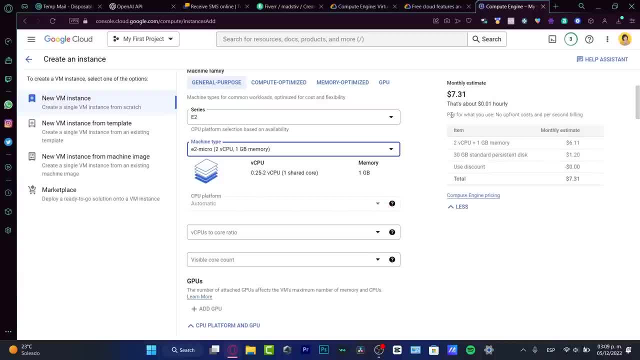 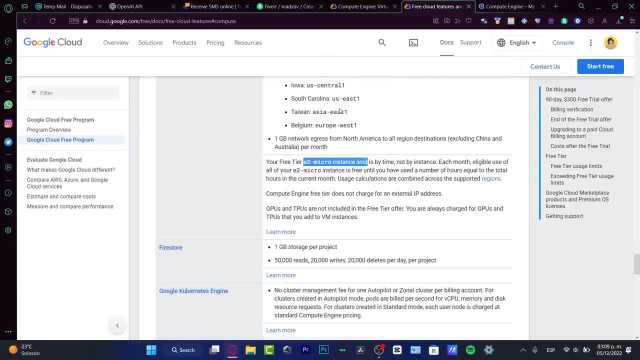 CPU has been added automatically. so once again, from twenty dollars this has been low to seven dollars. so that's what we're doing here, once you actually don't pay for actually anything. now the compute engine free tire does not charge for an external IP address, so you can add that if you wanted to. so the GPO and 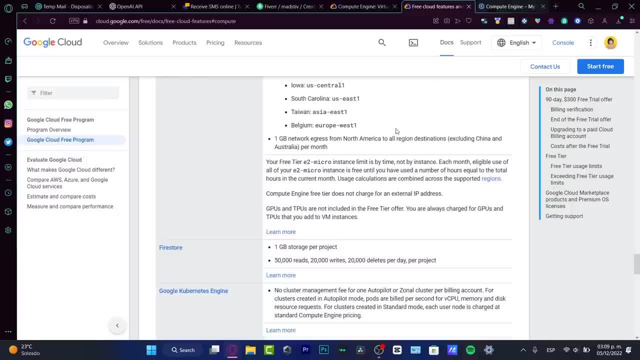 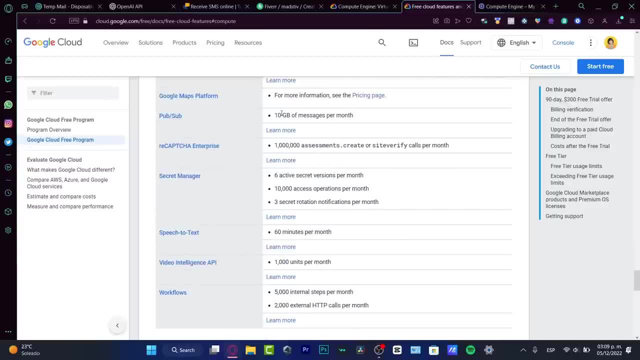 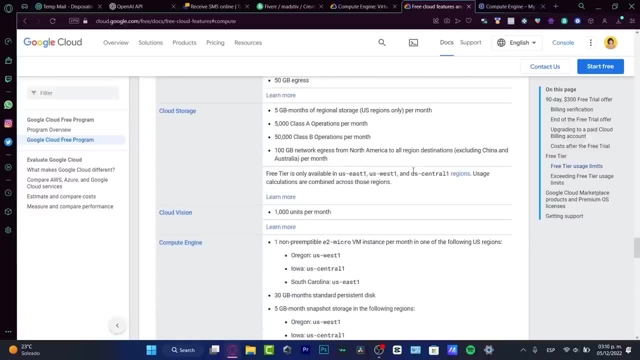 TPU are not included in the free tire offer. I'm going to hit into the one storage per project. one gigabyte storage per project, all right, we do have a 10 gigabyte of messages per month, which I think is really, really awesome, because this is like a free version, right? so in? 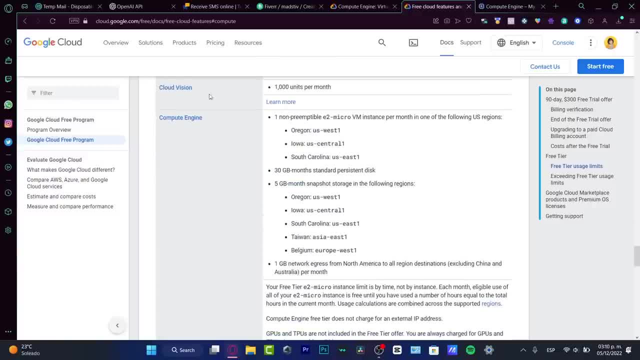 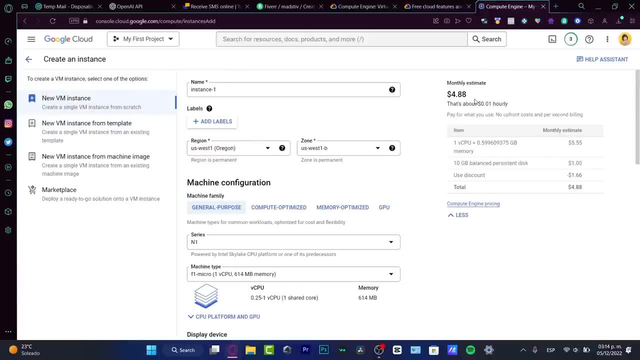 the cloud storage. if you want to change that, you can do that, but if we're just focusing into the compute engine, so what we did here is to change up to every tree was like thirty dollars, something like that. we just go low from thirty dollars into four dollars and we do have the 19 days for free of. 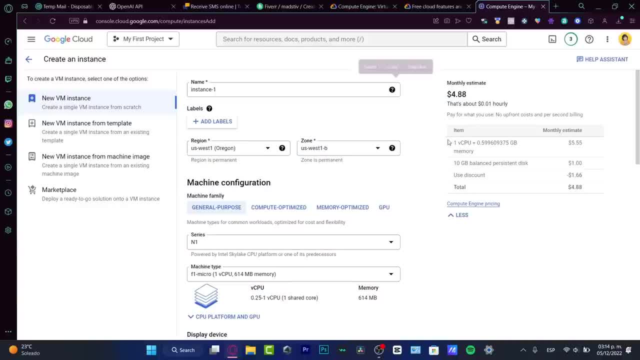 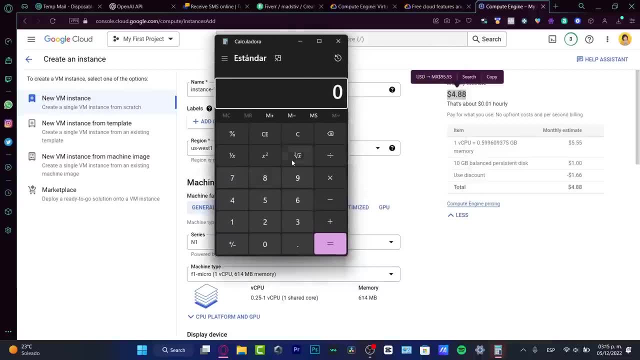 the three hundred dollars, which this is the only estimated thing. it's gonna be helping me a lot for the annual plan, so I'm gonna hit into my calculator and go into the four times 12: 58. I mean it, it's more than enough. I think it's really.